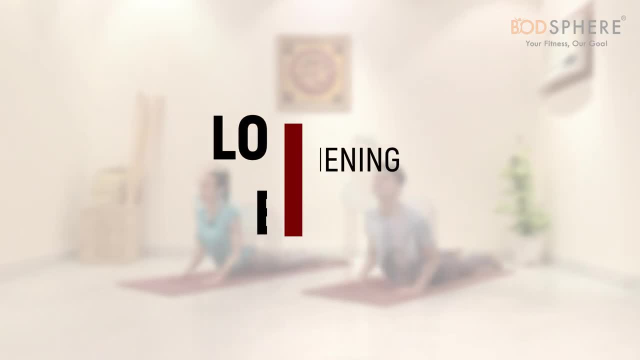 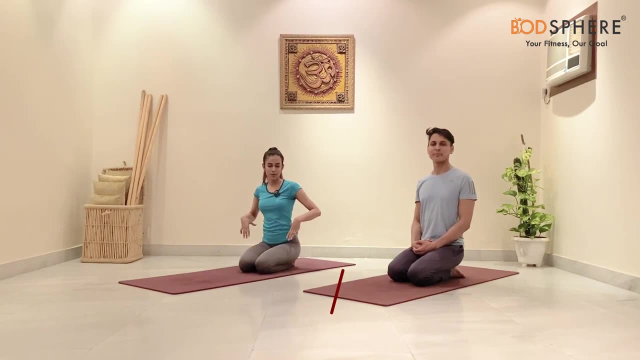 Hi, I am Pritika and he is Samarthya, So today we both are here to make a short video on lower back strengthening arsenals, which is very much in demand and a lot of people have requested for this. So this is due to poor posture, soft mattress or unhealthy lifestyle. 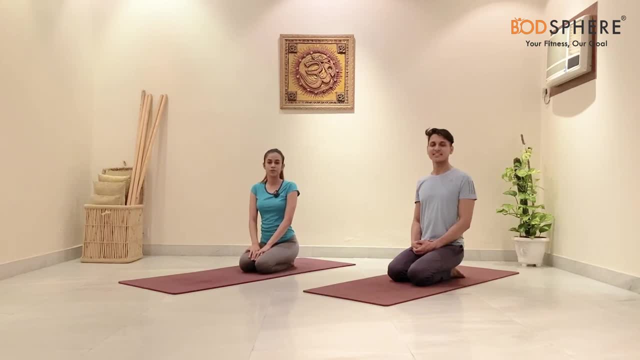 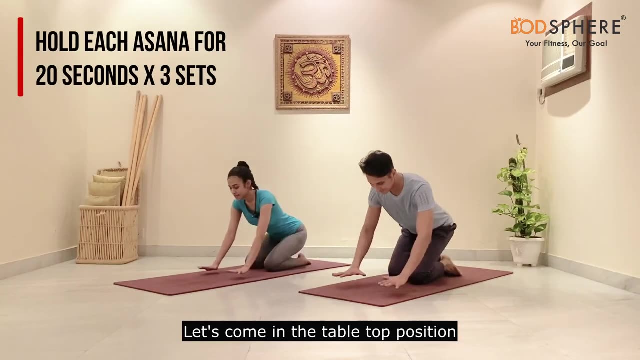 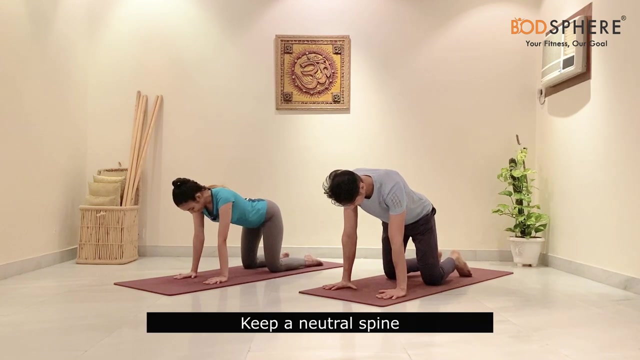 So we will be showing some lower back strengthening arsenals, which will be very effective for you guys. So let's get started. So now let's come into our first pose, that is, tabletop position. Your shoulders should be right above your wrist. Your spine should be neutral Hips. 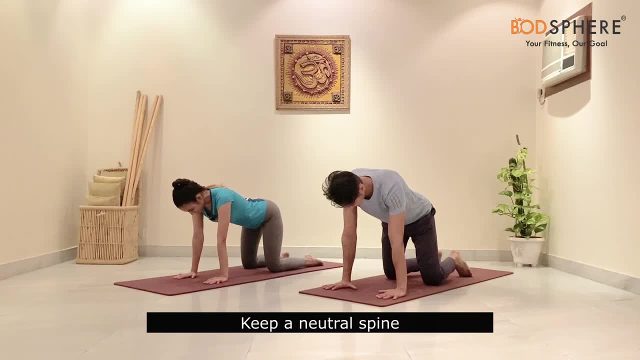 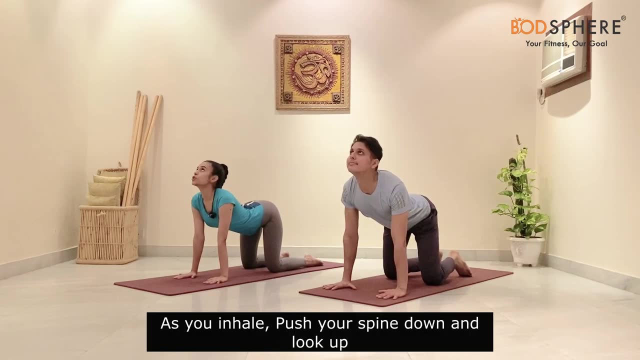 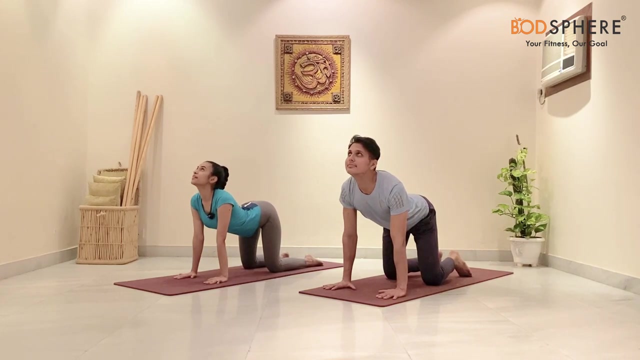 should be in line with your knees. And now let's inhale, Let's scoop our spine in, Let's come in cow pose, Look up, Push your lower back, middle back in towards the floor And your pelvic region is engaged. and in Let's hold the asana And keep inhaling and exhaling. 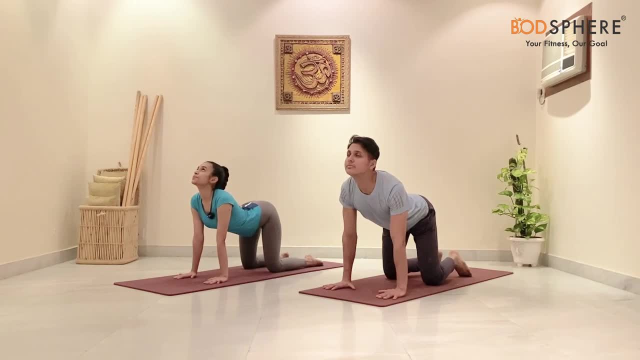 In the posture. Inhale And as you exhale, let's come in cat pose. Engage your scapula, your shoulder wings, Your middle back is pushed up. Look in Towards the thighs And keep inhaling and exhaling in the posture. Let's hold the posture. 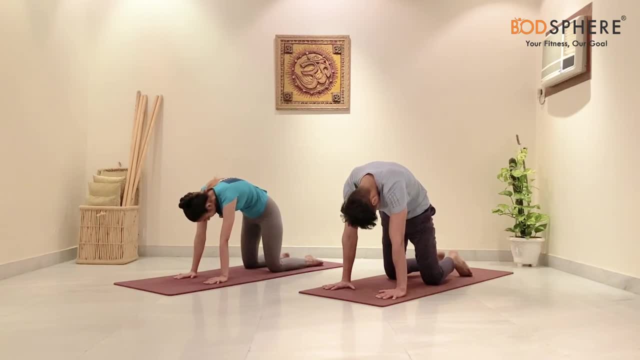 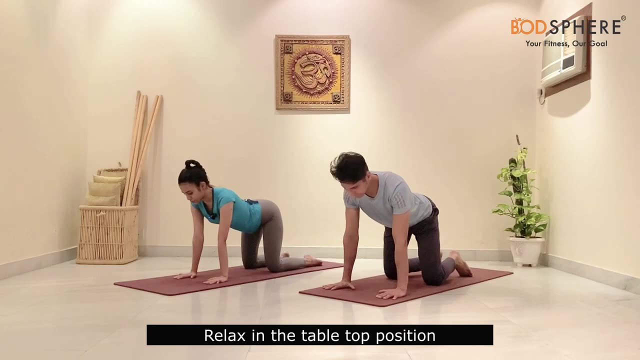 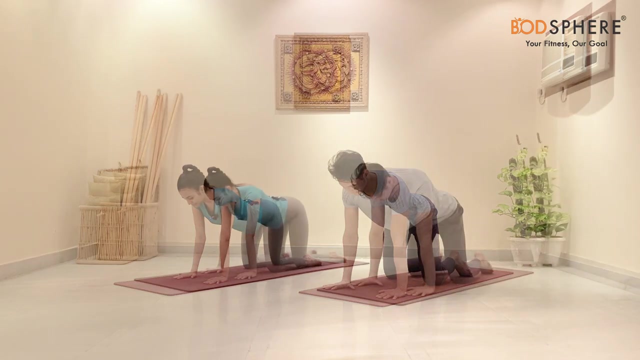 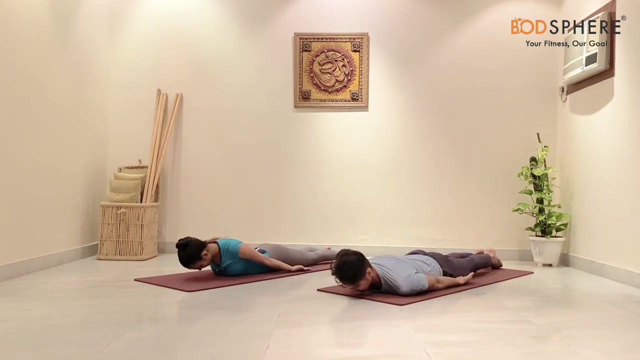 for a few seconds And as you inhale, let's come back to tabletop position, once again with the neutral spine, And relax. So from here now, let's lie down on our belly Arms by your side, Keep inhaling and exhaling in this posture, Breathe normally And just relax your whole. 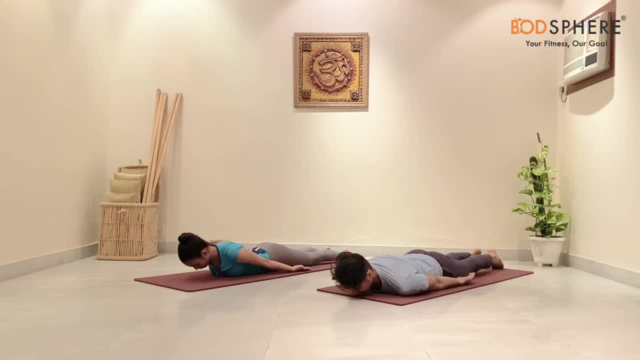 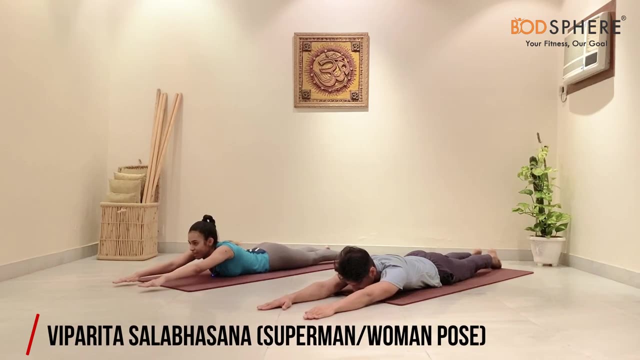 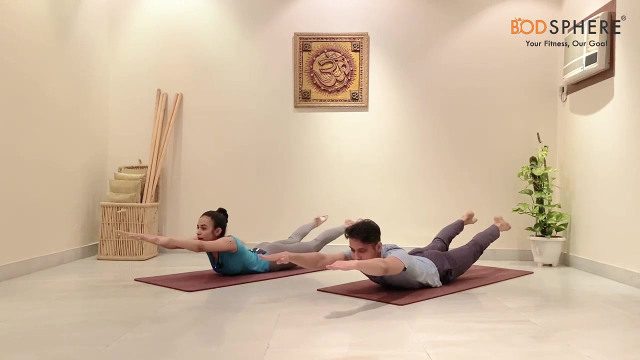 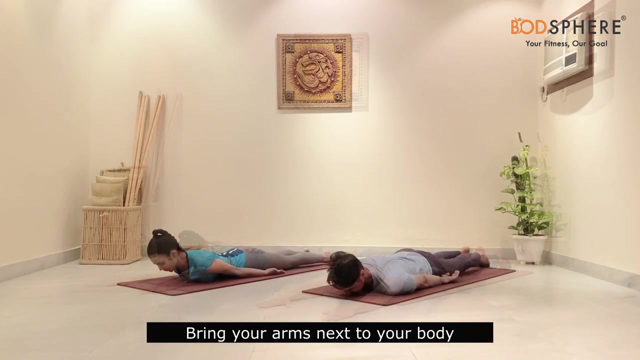 body. Now let's get ready for the superman pose. Let's take our arms in front And let's inhale. And let's take our legs and arms up, Hold the Asana for few seconds, Look in front, engage your back and hold and, as you exhale, relax. So now let's 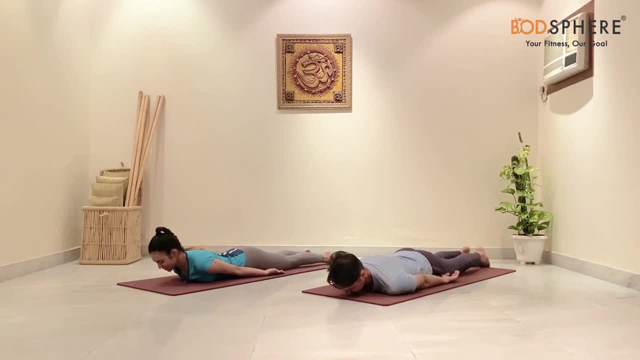 come into half locus pose. So let's make a fist with both the hands and let's place them under your groin region and now inhale. take your right leg up. Let's hold the asana for a few seconds. Keep breathing in the asana. 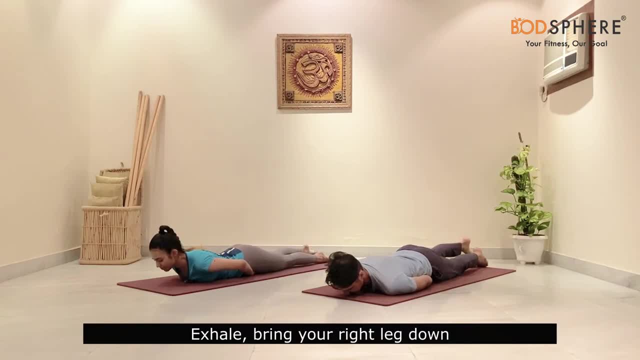 and, as you exhale, relax your leg and now inhale. let's do it for the other leg. You can take your left leg up and let's hold. Keep breathing. hold for a few seconds and, as you exhale, bring your leg back. Keep your hands down under your groin. 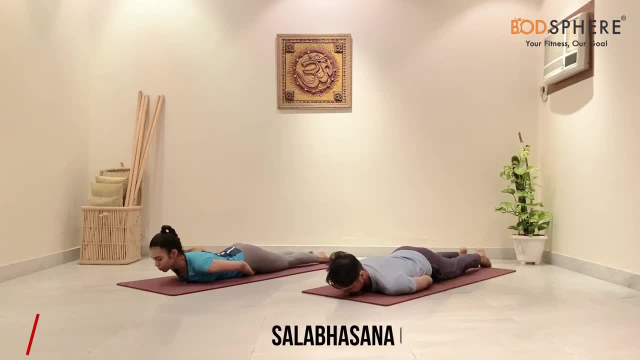 region. Now let's get ready for the locust pose. Let's inhale and let's take both the legs up. Hold the asana for a few seconds, Keep inhaling and exhaling. Your both the legs are up, your lower back is engaged, your glutes are engaged. 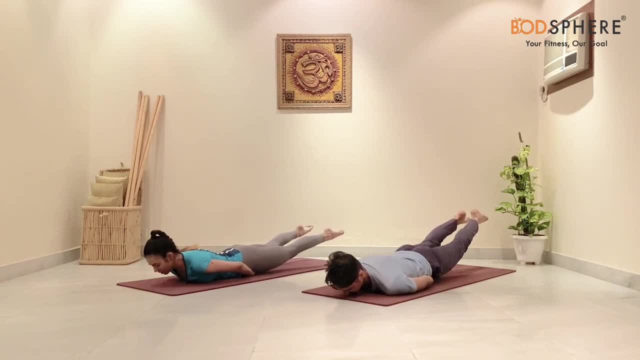 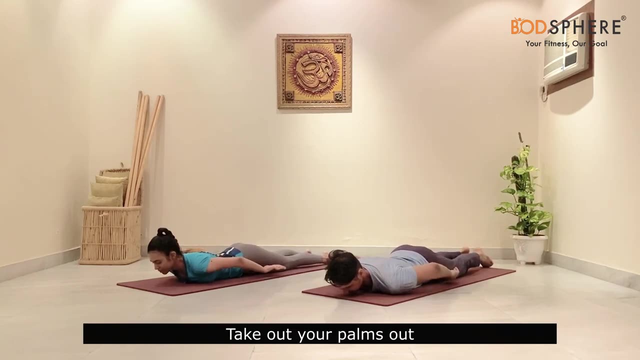 And, as you exhale, relax your legs. You can relax your hands. You can open up the fists And relax your body down on the floor. Now let's get ready for the Bhajung Asana. You can bring your palms near your chest. 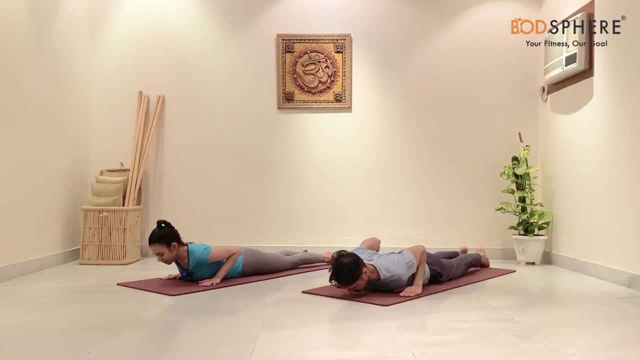 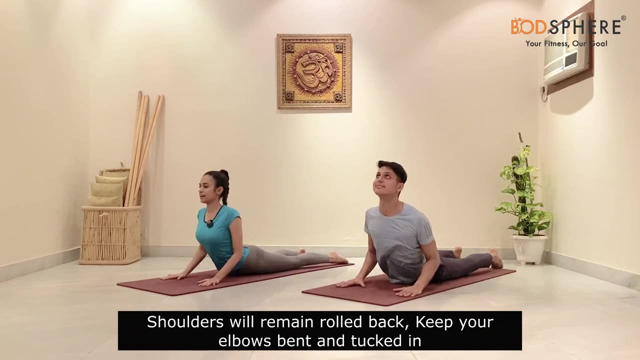 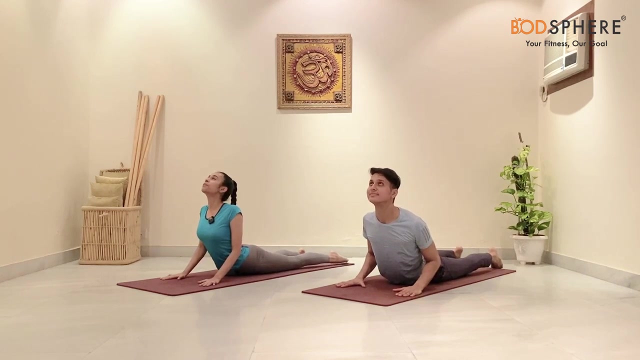 Place your hands near your chest, Inhale, take your upper body up your lats with your left leg to the ground. feet face forward around the ACT up navel one inch above the ground. your elbows are bent and tucked in, shoulders are relaxed and rolled back. you can inhale and look up. keep breathing in the 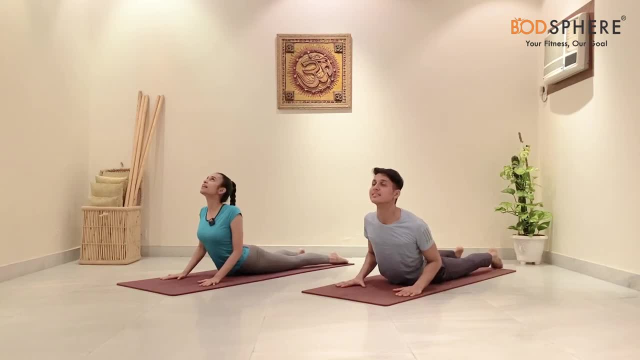 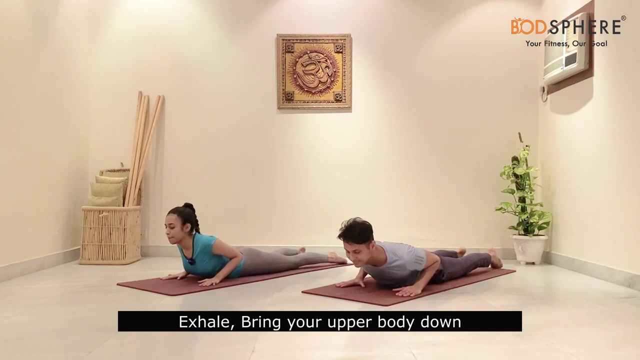 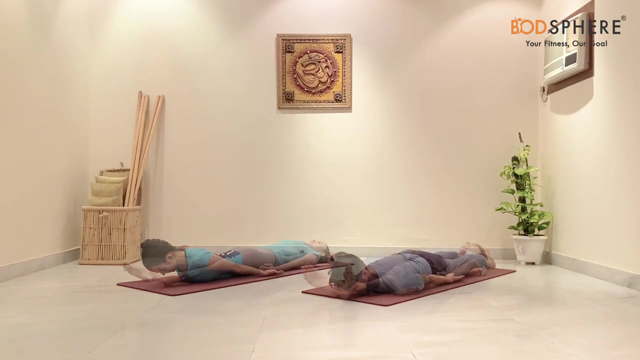 posture, keep inhaling and exhaling and as you exhale, you can come down, come back, you can relax your hands and relax the whole body. now for the last asana. let's lie down in shavasana and let's get ready for the setu bandhasana. you can fold your legs, you can. 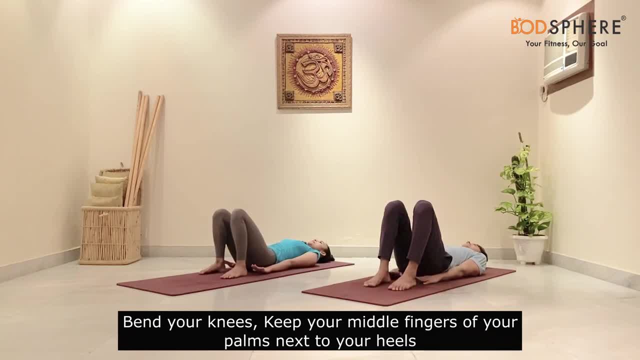 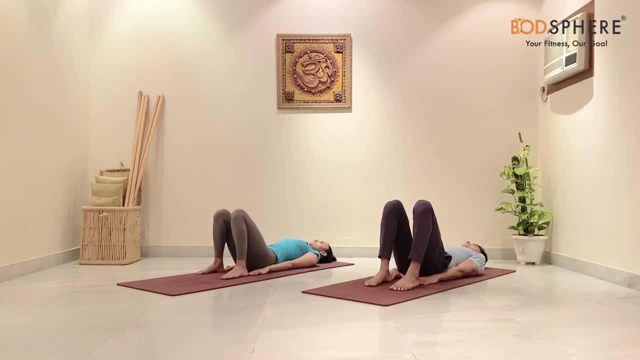 middle finger with your heels and, as you inhale, take your buttocks up, lower back up. keep pushing your lower back and your buttocks up towards the ceiling. keep inhaling and exhaling. let's hold for few seconds and, as you exhale, bring your buttocks back me start slow down, keep your goose bumps. 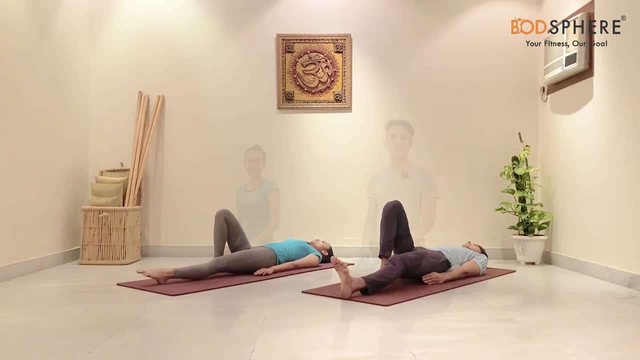 relax your legs, you can come back to shavasana, so this video was all about lower back strengthening asanas. I hope you liked the video. of course, there are a lot of asanas which you can do just to strengthen this area or the lower back, and if you have any questions of any sort, whether it is, 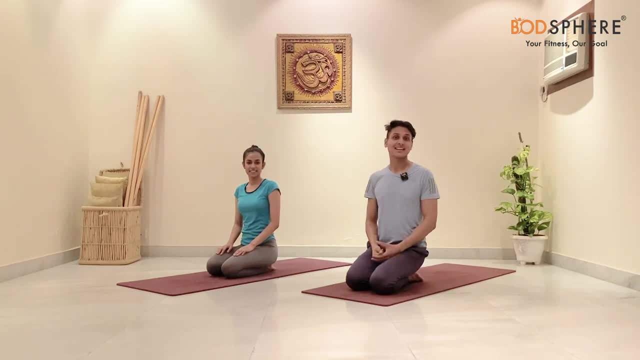 yoga, or mind light, or self called awareness. yoga also has so many things to do. when in itself love the anger emotions of which you can least enjoy влиing on yourself meditation, fitness, health or life or spirituality in general, we are always there with you and if you have any questions or queries, please don't hesitate to write down in. 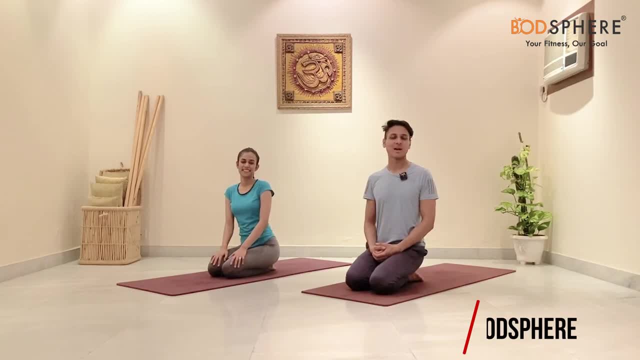 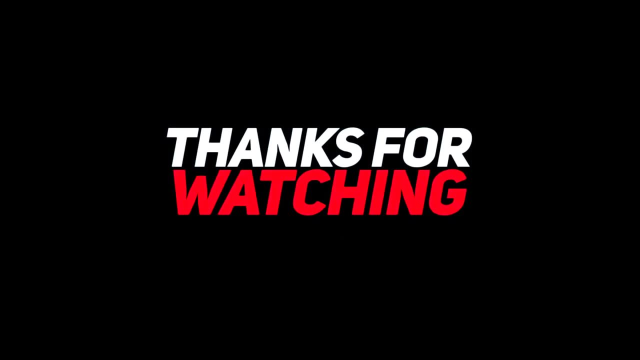 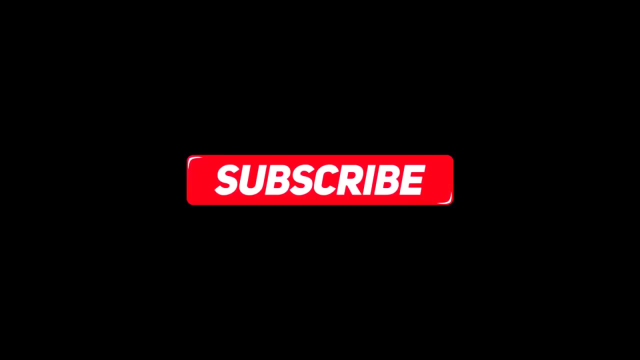 the comment section below, and please don't forget to subscribe to our youtube channel, namaste.